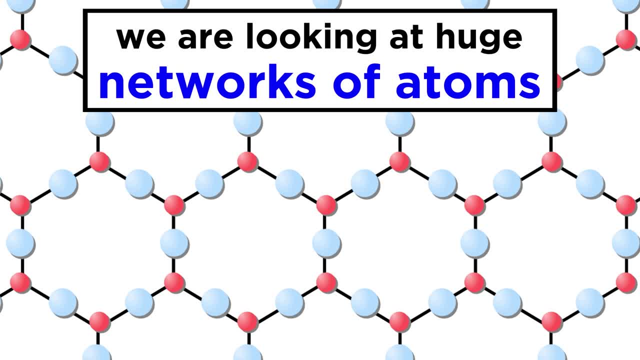 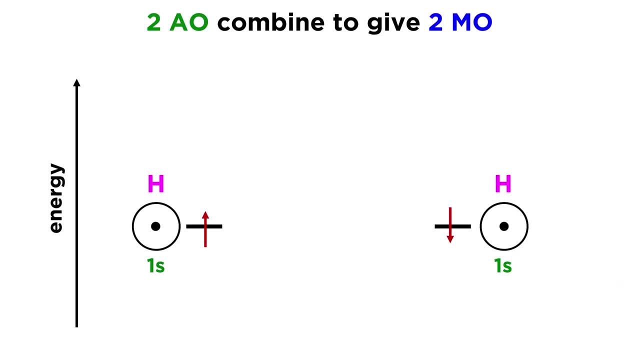 These are huge arrays of a particular atom or repeating formula unit, stretching the atom endlessly in every direction. We know that when two atomic orbitals combine, two molecular orbitals will be generated: one lower-energy bonding orbital and one higher-energy antibonding orbital. 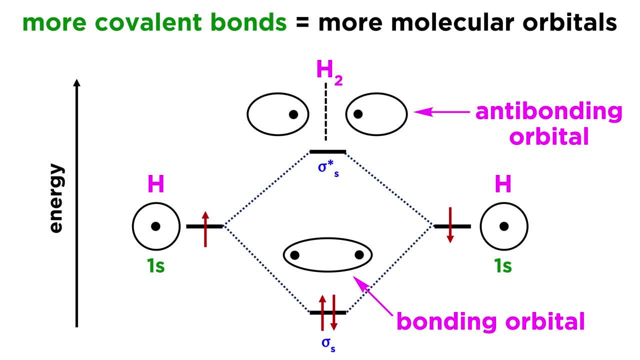 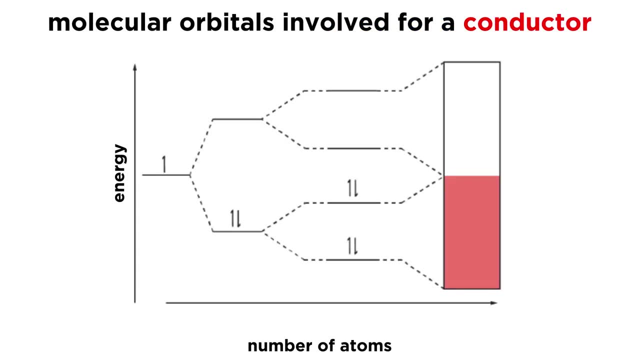 Thus, as more and more covalent bonds form, more molecular orbitals will be generated to house all of these electrons. Here we can see the molecular orbitals involved. As many atoms come together to make a network solid, that will be a conductor. 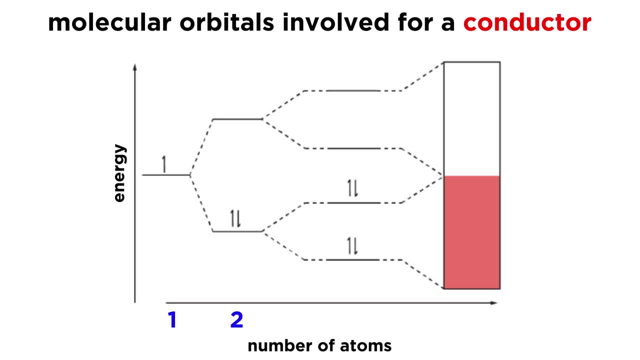 As the number of atoms increases from one to two to four, to a number so large that it can be compared with infinity for practical purposes. the number of orbitals will increase in the same way, and as the number of orbitals becomes incredibly large, they will begin. 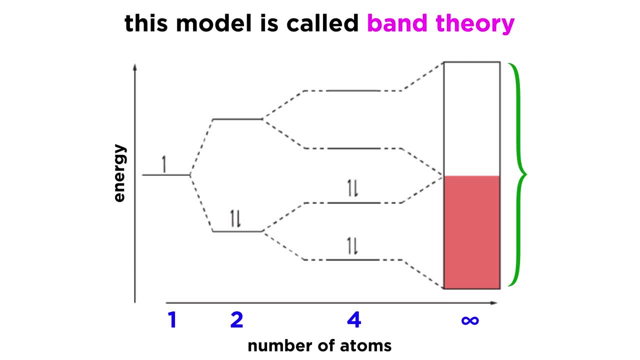 to resemble one continuous band. There are some important things to note about this model. First of all, the number of atoms will increase. There are some important things to note about this model, which we call band theory. First, the atoms are held together by electrons in the lower-energy bonding orbitals, as these: 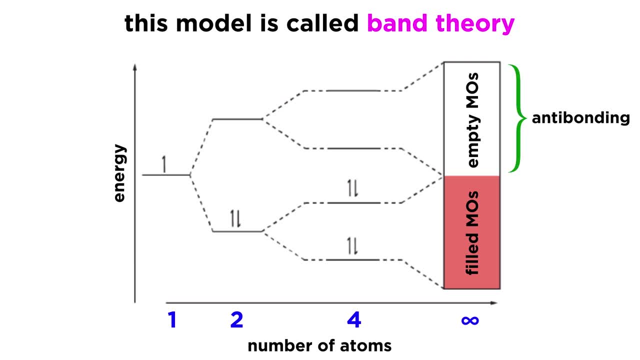 are filled, first, while the higher-energy antibonding orbitals remain vacant. Second, in a conductor, the difference in energy between the highest occupied molecular orbital and the lowest unoccupied molecular orbital is infinitesimally small, which means that electrons can move freely between orbitals, and this is the key feature of a conductor. 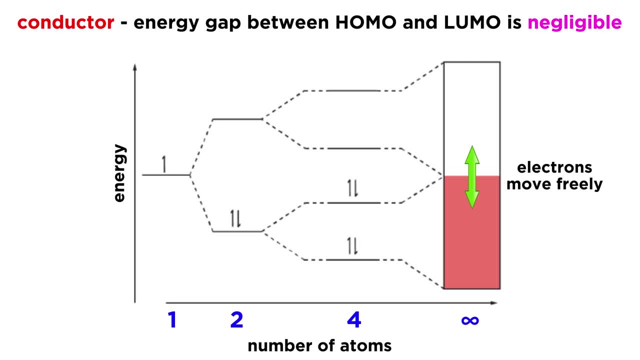 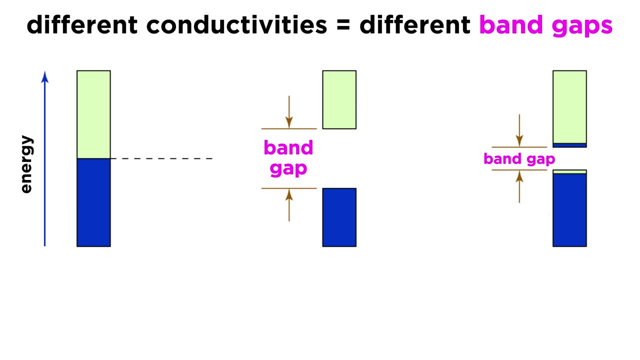 that allows it to conduct electricity. Comparing substances with differing conductivities, we will notice something called a band gap, which is a gap in energy between the bonding orbitals, or valence band, and the antibonding orbitals, or conduction band, named as such because electrons must access electrons as 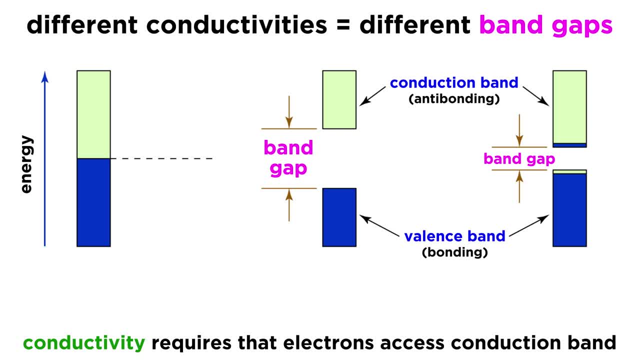 a result of the bond, these orbitals, in order for the substance to conduct electricity. Conductors, as we said, have no band gap, or just a tiny one, so electrons can flow easily. Insulators have large band gaps, which does not allow for a current to form. 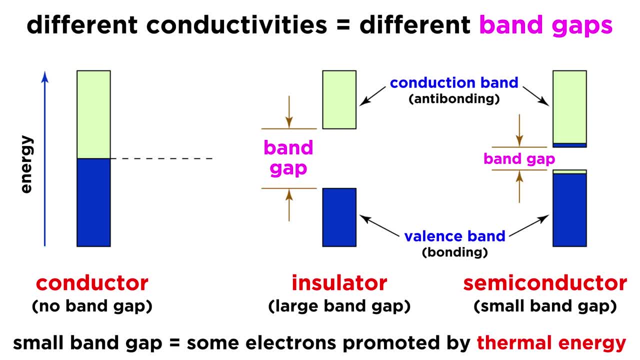 Semiconductors, on the other hand, have a small enough band gap that thermal energy in the system is able to keep some of the bonding orbitals in the valence band empty and promote some electrons into the antibonding orbitals in the conduction band. 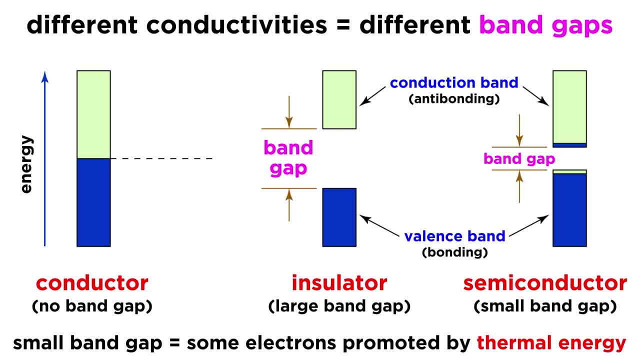 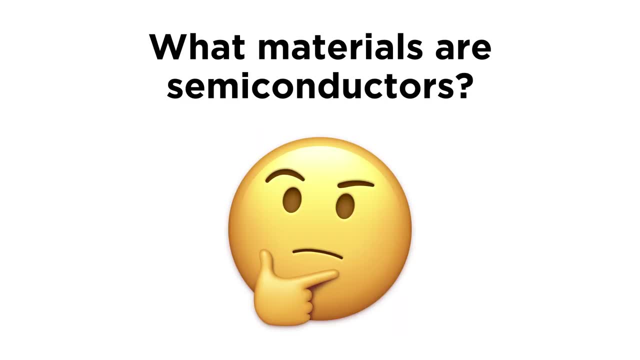 This is why semiconductors conduct electricity better at higher temperatures, because there is more thermal energy available to promote electrons into the conduction band and thus a stronger current is able to form. So what kinds of materials do we need? Most materials can act as semiconductors. 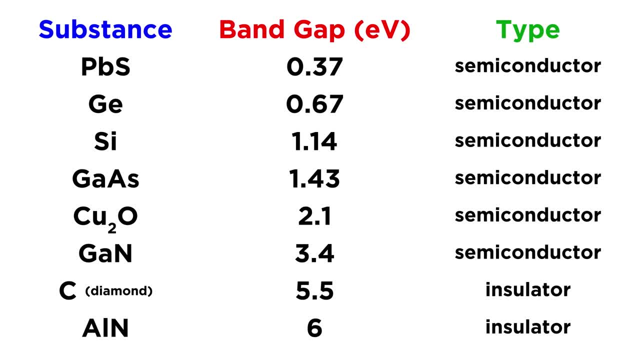 Here are some common substances, along with their respective band gaps in electron volts, so we can get a sense of the range that is permissible. We will notice that some of these substances are elements like silicon and germanium and some are compounds like lead sulfide. 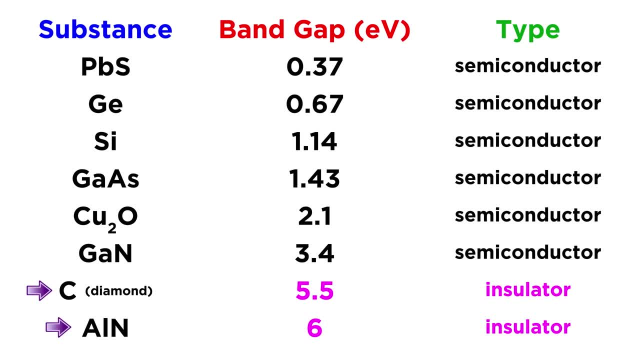 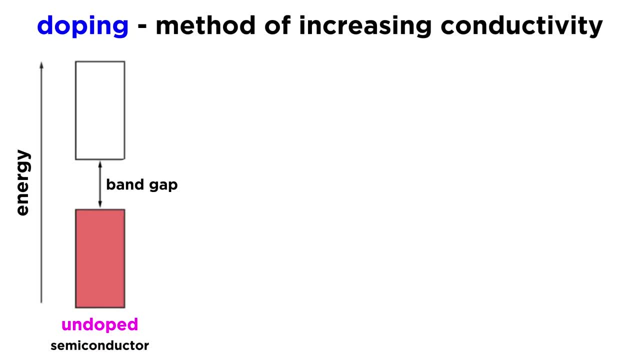 Once the band gap becomes sufficiently large, a substance will become an insulator like diamond or aluminum nitride. Apart from temperature, another way to increase the conductivity of a semiconductor is through a method called doping, which is where impurities are mixed into a substance, and this impurity 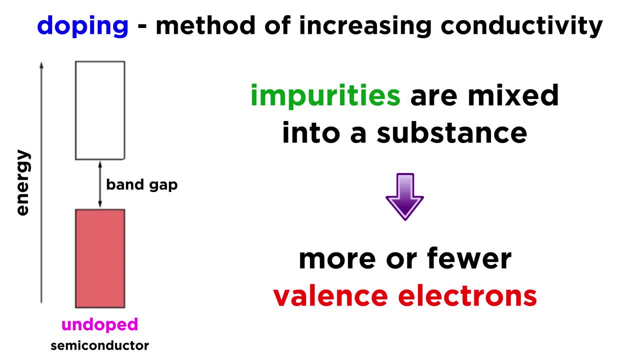 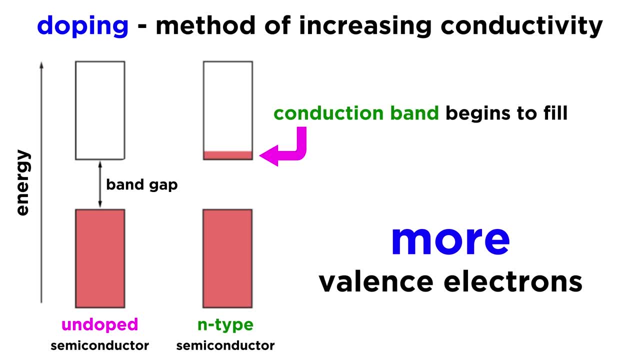 can either have more or fewer valence electrons than the substance. If the impurity or dopant has more valence electrons, the conduction band will begin to fill and current can flow. This is called an endoplasm. This is called a n-type semiconductor, where n stands for negative. 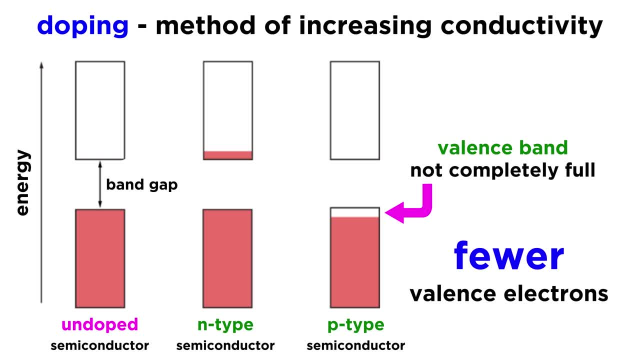 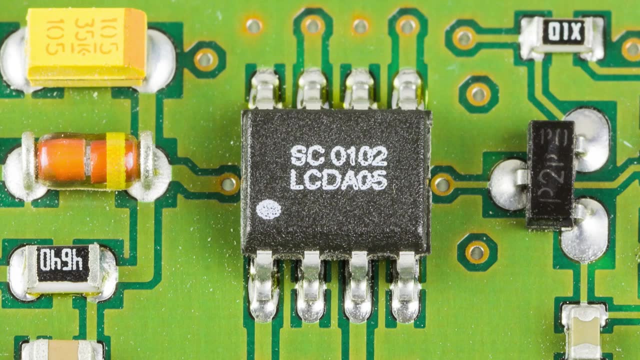 If the dopant has fewer electrons, the valence band will end up not completely full and current will again be able to flow. This is called a p-type semiconductor, where p stands for positive Electronic components like diodes and transistors utilize both p and n-type semiconductors.